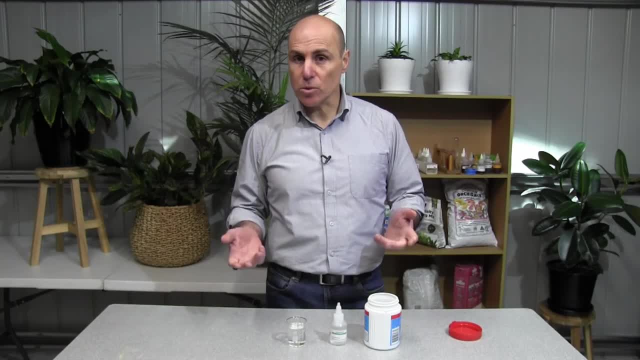 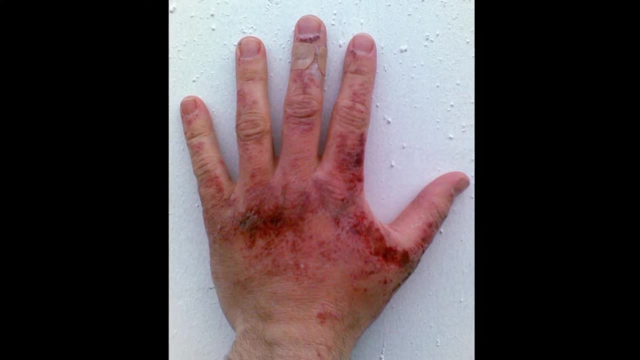 and textiles. It doesn't chemically react with metals, but it does chemically react with proteins and fats, so it should be treated with caution. It can cause severe chemical burns on your skin, so you have to be very careful. The sodium hydroxide in this beaker. 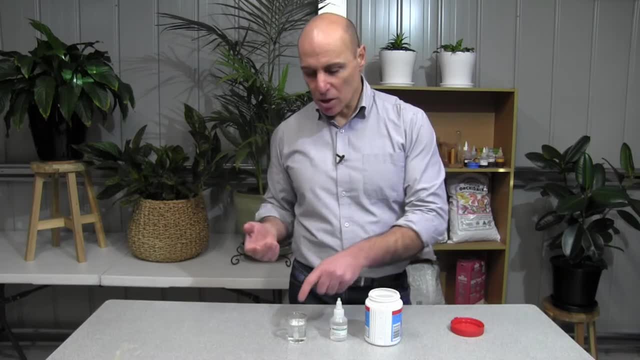 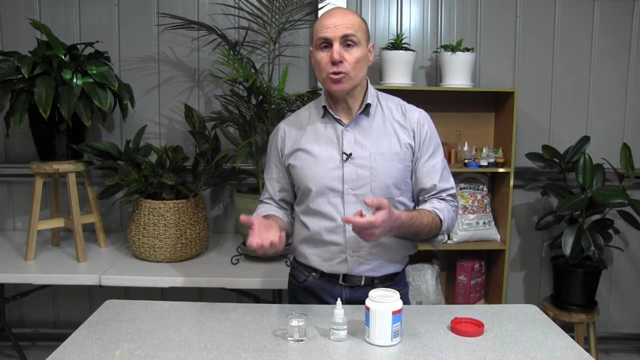 is heavily watered down. so even if I touch it- which I shouldn't really do, it doesn't really do much damage. But if you do get any on yourself, you should try to wash it off as soon as you can. It kind of feels soapy because it chemically reacts with the oils. 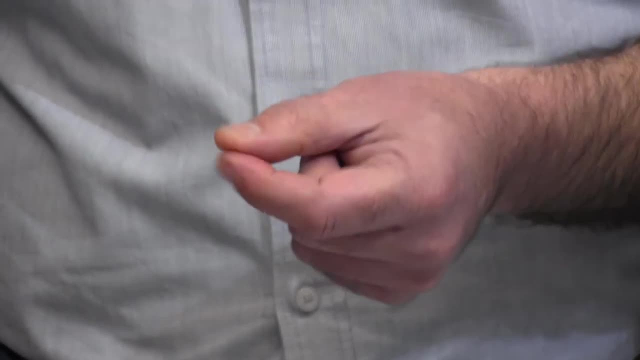 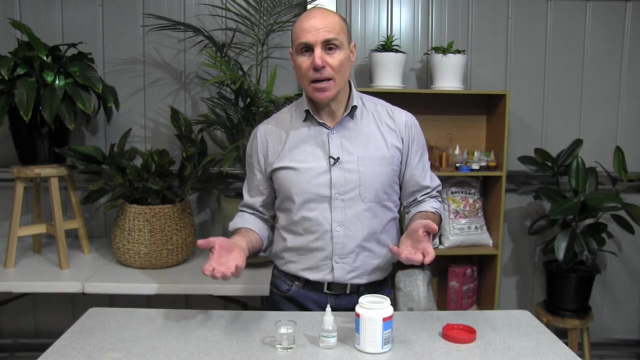 on my skin and turns them into chemicals that are a little like soap, Like the chemicals in soap. As watered down as this is, if it gets into your eyes it can do major damage. So again, be careful If you've ever felt the sting of soap in your. 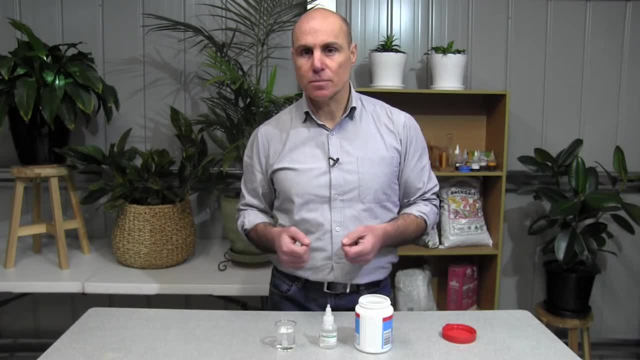 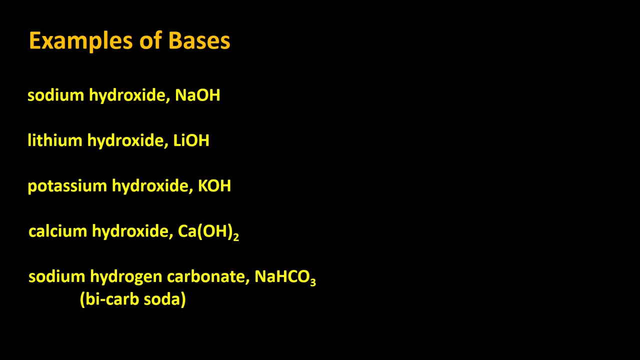 eyes. getting this into your eyes is much, much worse. Bases are hugely important in lots of industries. For example, sodium hydroxide is used, as I said, in the production of soap, paper and textiles. Lithium hydroxide is used to produce 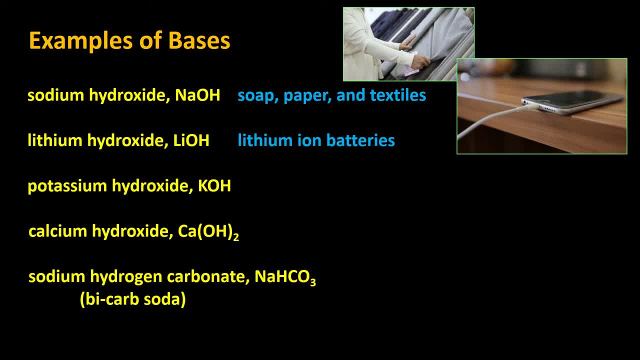 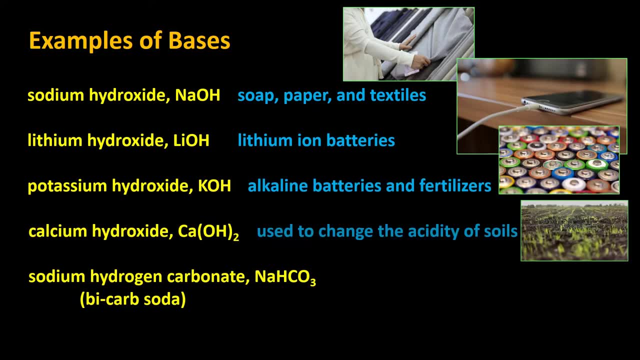 lithium ion batteries in phones, computers and electric vehicles. Potassium hydroxide is used to produce alkaline batteries and fertilisers. Calcium hydroxide is used to change the acidity of soils on farms, And sodium hydrogen carbonate- bicarb soda, which we looked at extensively in our last. 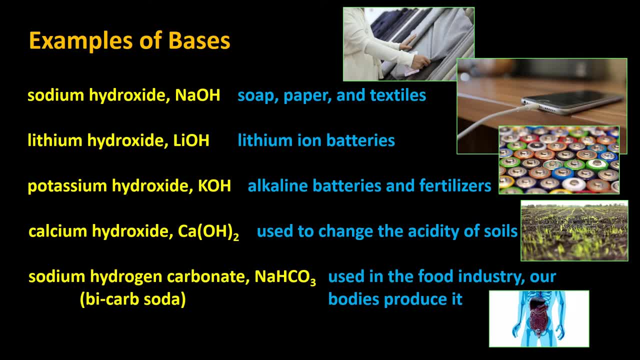 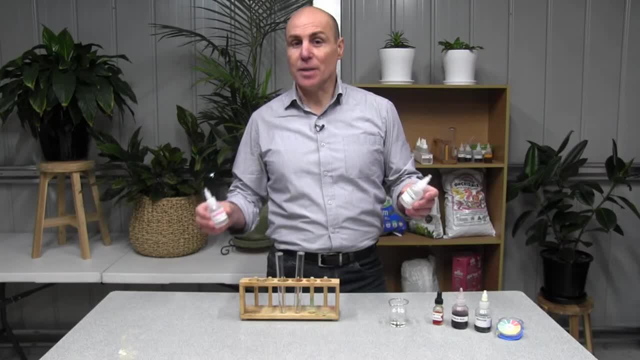 episode is used in the food industry a lot and our bodies produce it to neutralise the stomach acid that enters the small intestine At a basic level- pardon the pun, I should say at a simple level. a base is a chemical that reacts with an acid. 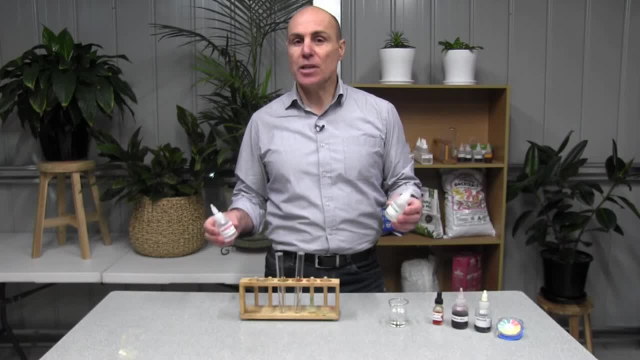 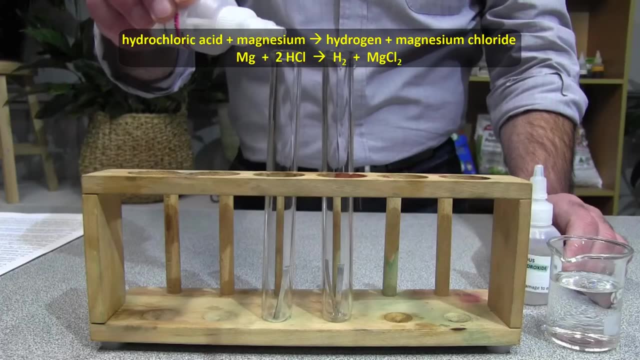 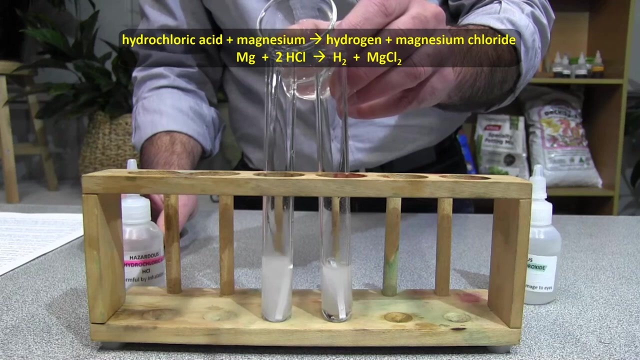 This reaction is called a neutralisation reaction, because the acid and the base neutralise each other. Let me demonstrate: As we've seen, hydrochloric acid reacts with magnesium, and that's what's happening in these two test tubes. Now, if I pour water into the test tube on the left, I water down. 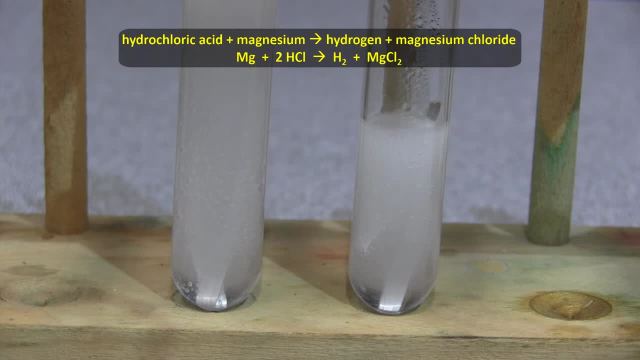 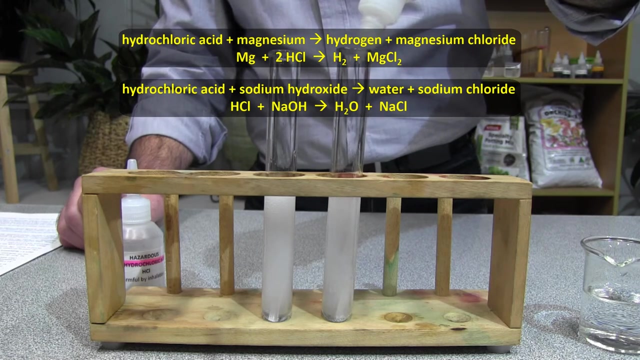 the acid even more than it already is. That is, I'm diluting the acid even more than it already is, And so the reaction slows down a little, but it continues because the acid is still there. Now, if I add some sodium hydroxide, a base, into the test tube on the right, the hydrochloric 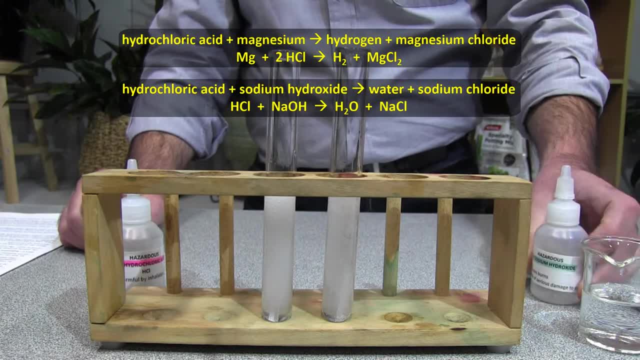 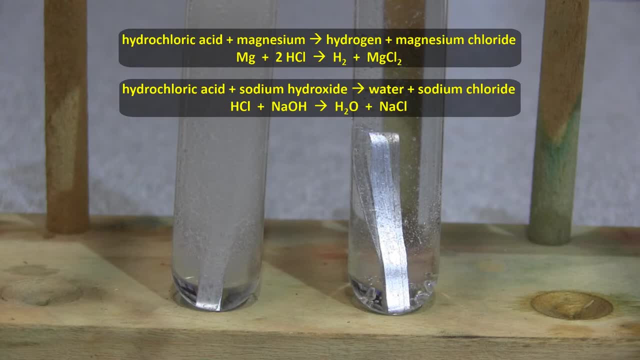 acid immediately reacts with it and water and sodium chloride are produced. The Mg is not producing bubbles anymore, because there is literally no acid in the test tube anymore. The acid has chemically reacted with the base, so now I just have a piece of magnesium lying. 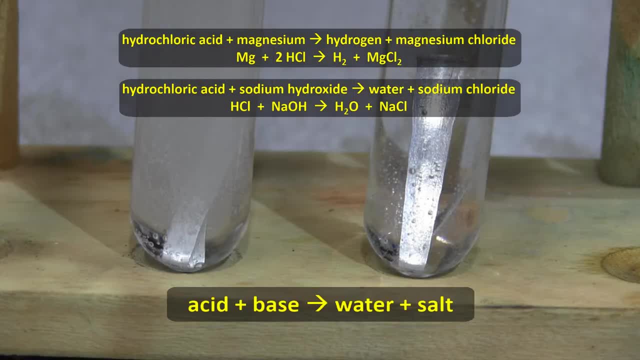 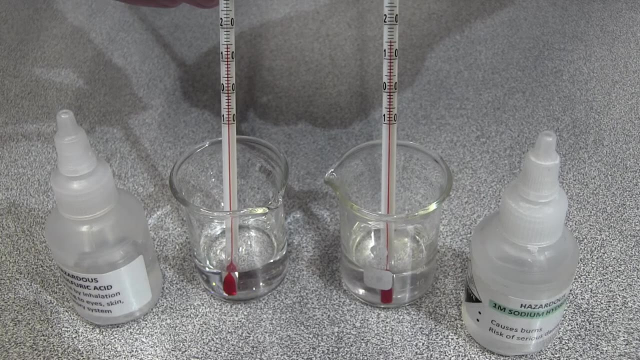 in a test tube that has water and salt in it. So, in general, an acid plus a base produces water, And this is called a neutralisation reaction. The mixture of salt and water is neither acidic nor basic. It's neutral. Now, when a neutralisation reaction occurs, it's not always obvious, but heat is always. 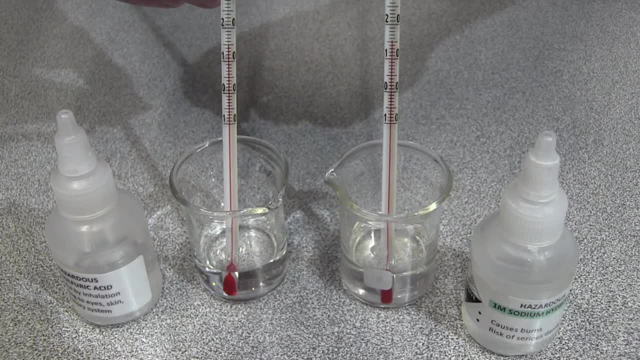 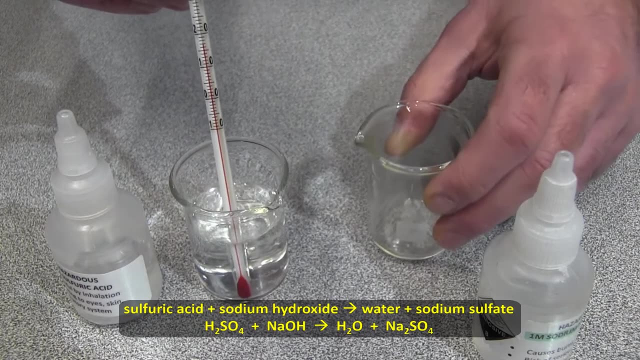 generated. The sulphuric acid and the sodium hydroxide here are both about 15 degrees Celsius, but when I mix them, a chemical reaction takes place which produces water and sodium sulphate and the temperature quickly rises to about 20 degrees Celsius. 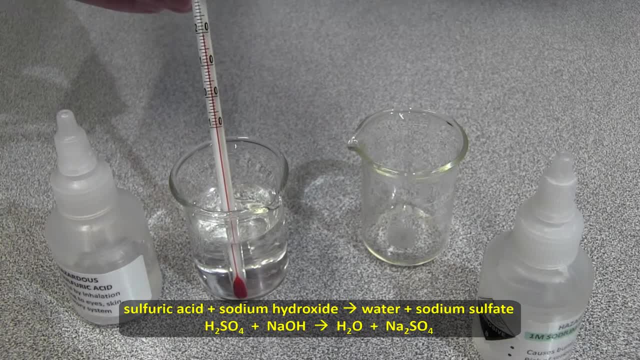 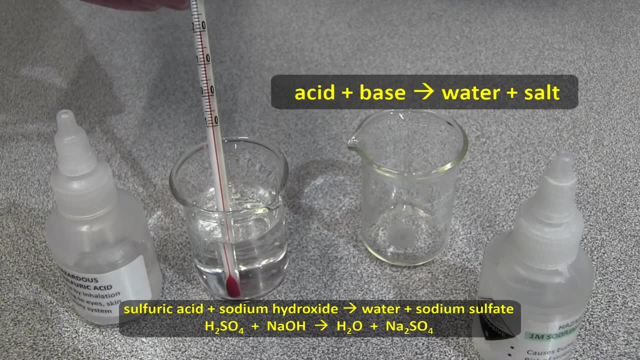 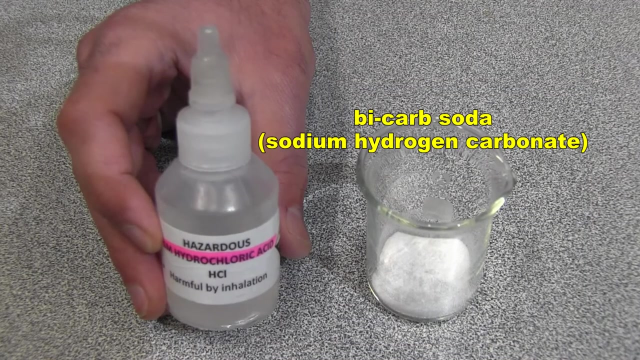 This temperature change tells us that a reaction has occurred, but, as I said, it's not obvious because the sodium sulphate remains dissolved in the water. Once again, the general equation holds, but the salt produced this time is sodium sulphate. Bicarb soda, that is, sodium hydrogen carbonate is also a base, If I add some hydrochloric. 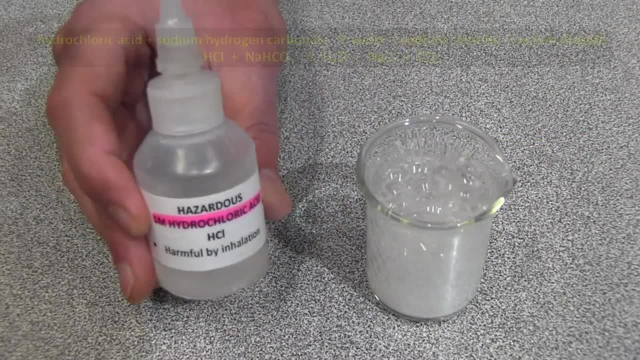 acid to the bicarb soda. they both neutralise each other. Hydrochloric acid plus sodium hydrogen carbonate produces water plus sodium sulphate. Now when I add some salt and sodium hydroxide, it's also a base. but if I add some sodium, 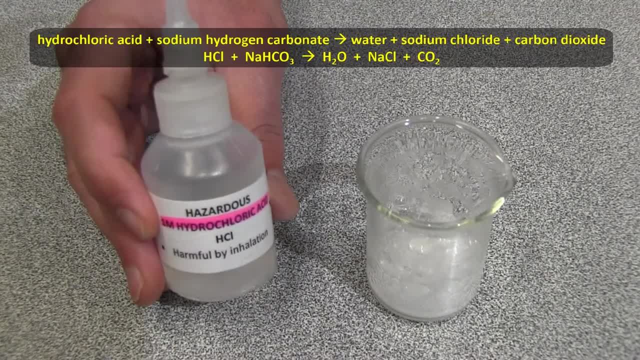 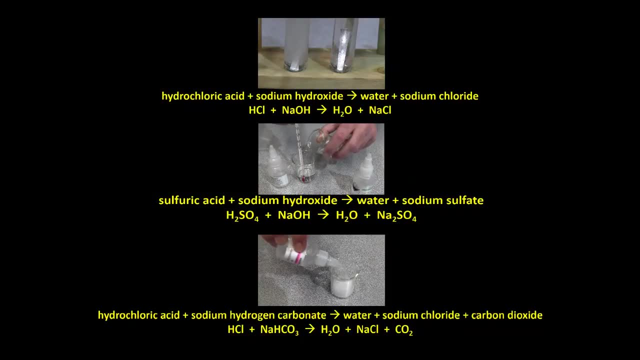 plus sodium chloride, a salt plus. this time we also get carbon dioxide, most of which just floats away. Now, in these neutralization reactions, what's left in the glassware may still be acidic or basic, because the amount of acid and base I added, and or how concentrated they were, may not have been. 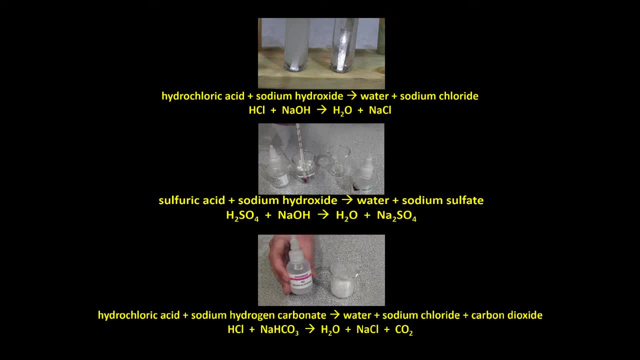 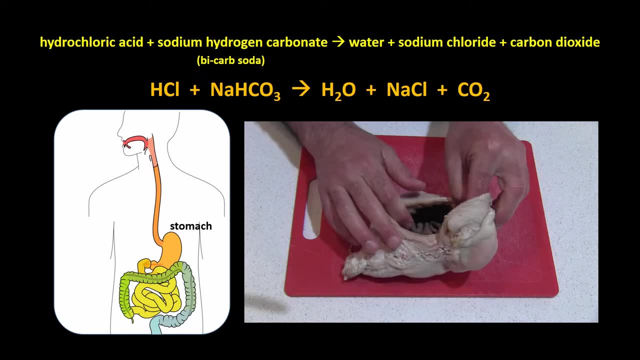 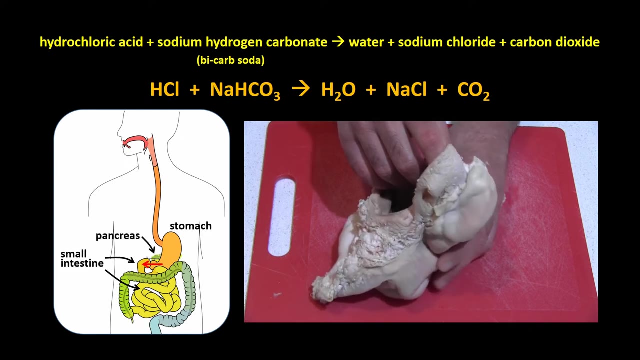 the same, Neutralization still occurred, but some acid or base may still be left over. In our last episode we saw that the stomach acid carrying the partially digested food that gets squeezed into the small intestine chemically reacts with the bicarb soda that is produced by our pancreas.